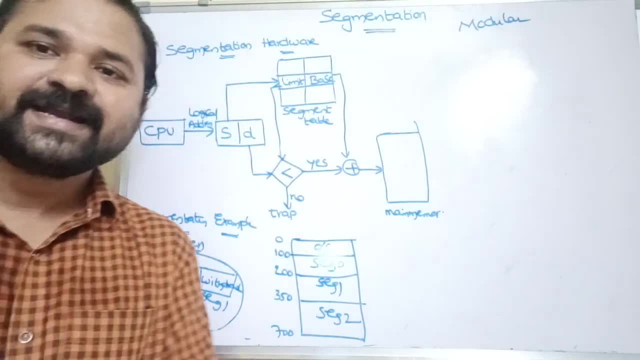 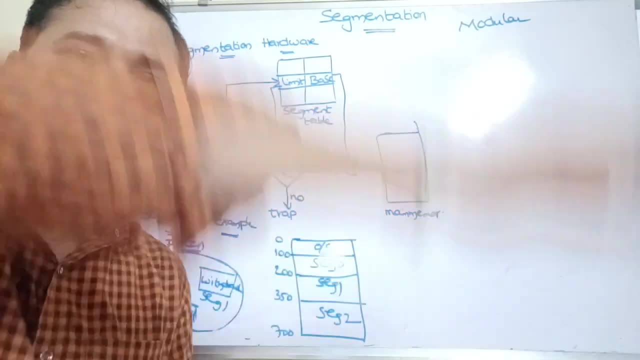 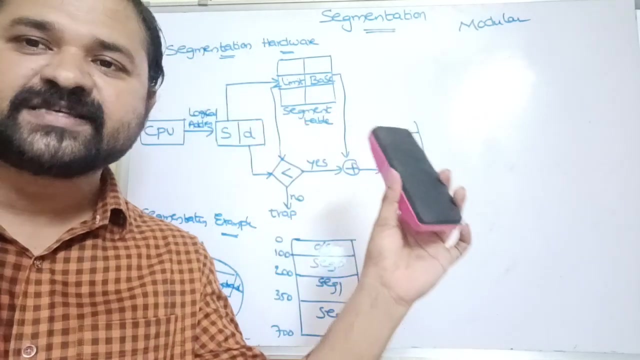 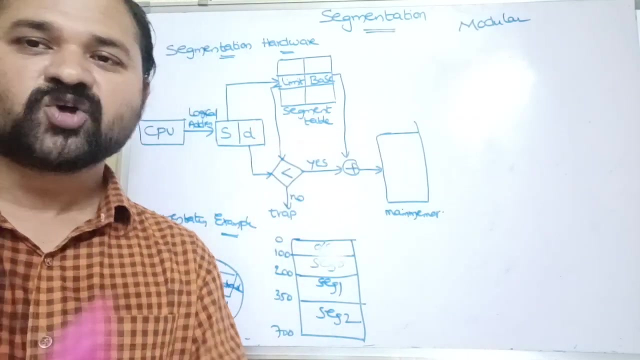 So what is the major problem with paging? It doesn't maintains modular structure. Same method may resides in multiple pages of the process and multiple frames of the main memory. So in order to overcome that problem, we use segmentation. So segmentation is a non-contiguous memory allocation, just like paging. So we know what is non-contiguous memory allocation. 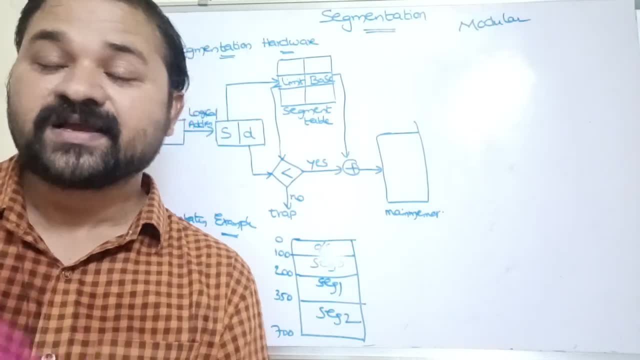 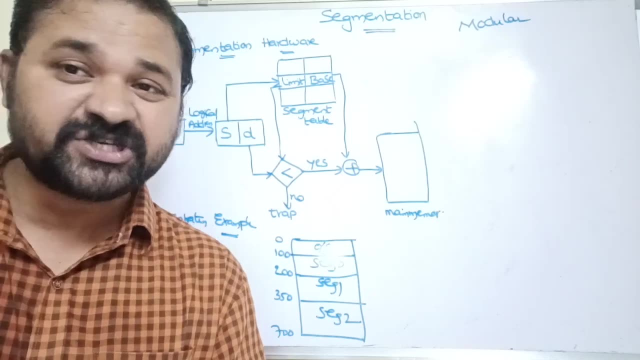 So segmentation is a non-contiguous memory allocation. So we know what is non-contiguous memory allocation. So now what will happen when the function is allocated for segmentation? Let's see what that function is placed in the following way: Whenever there is a free partition, then the non-contiguous memory allocation stimulate in the confront of the 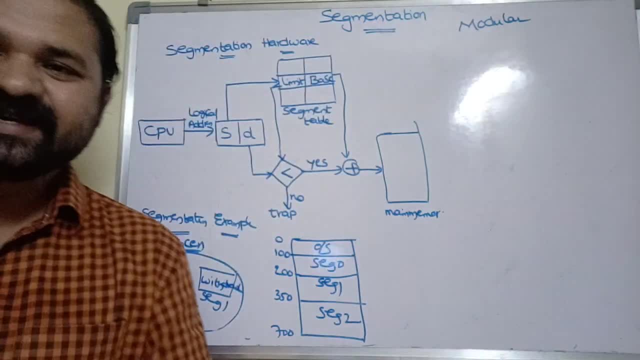 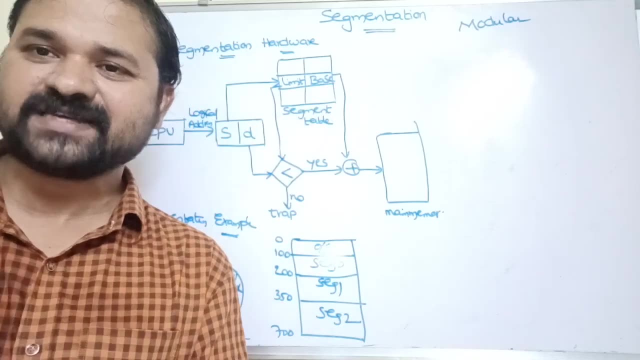 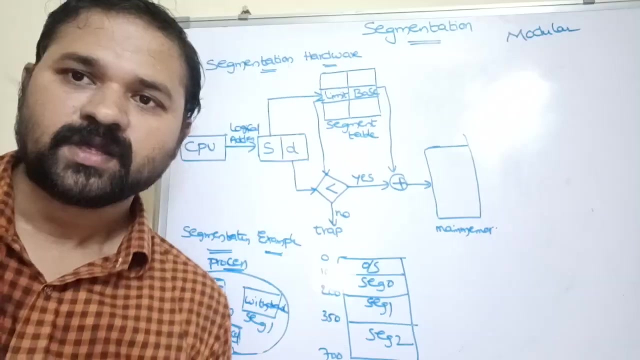 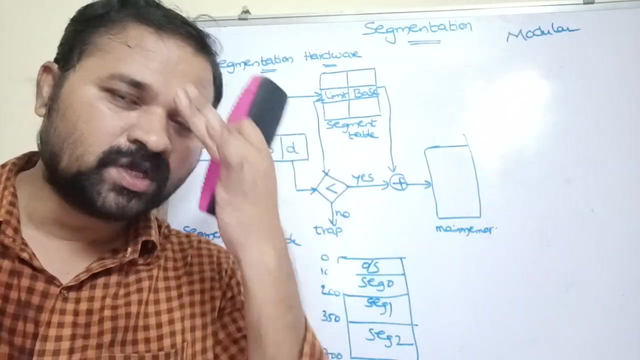 config promoting this function. Then the print messages are given. So the collection of statements, some Boolean performance. Now the condition for alevant execution is defined later. Here the memory allocation is assumed as a significant System is 我要 for the segments is similar to paging process only. So the given process is divided into. 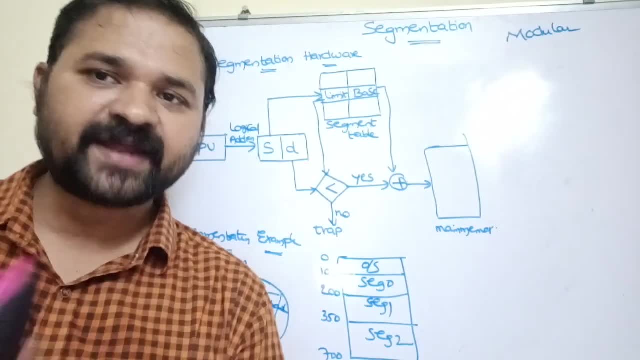 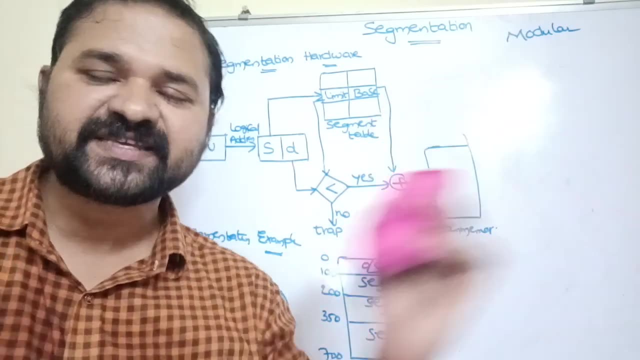 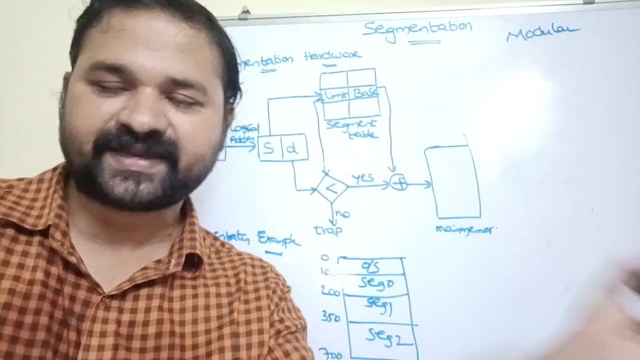 a number of partitions. But here the size of a partition is similar to the size of a segment. So the size of a partition depends upon the size of a segment. Suppose, if a segment size is 10 kb, then 10 kb of the partition will be allocated for the segment. Suppose, if a segment size is 30 kb. 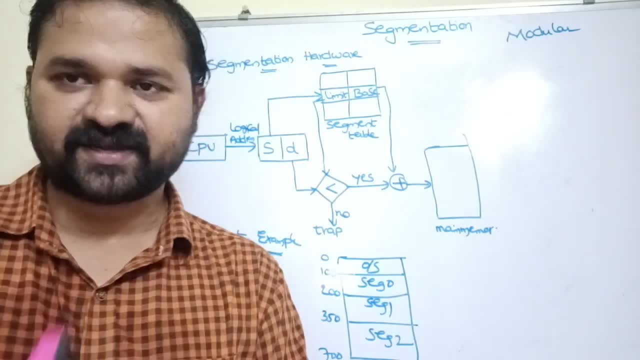 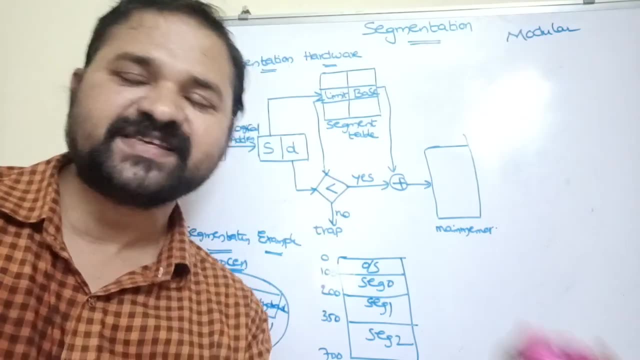 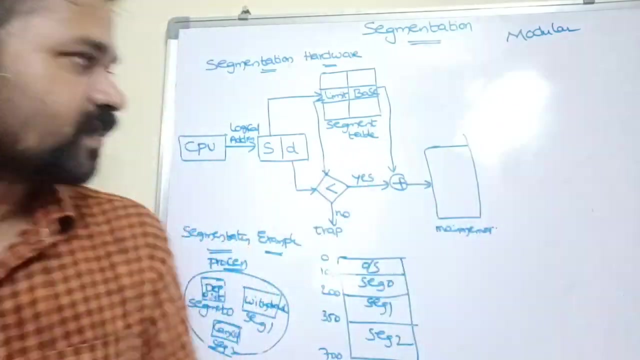 then 30 kb of the partition will be allocated for the segment. So likewise, the main memory is also divided into a number of partitions. that depends upon the size of the segment. So operating system allocates a free frame for the corresponding segment. Now let us see this example so that 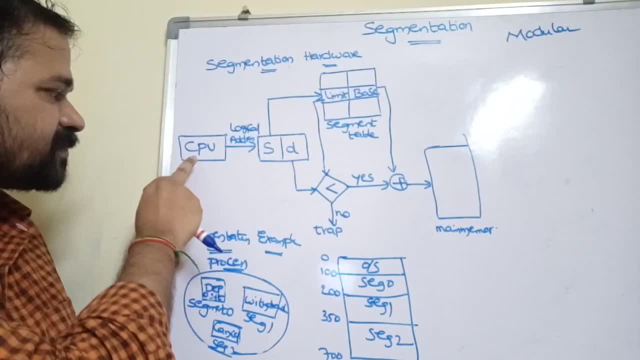 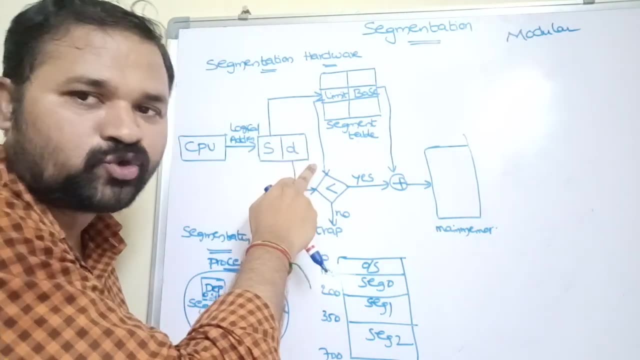 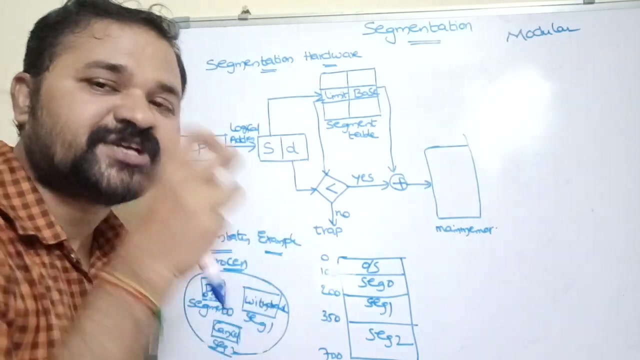 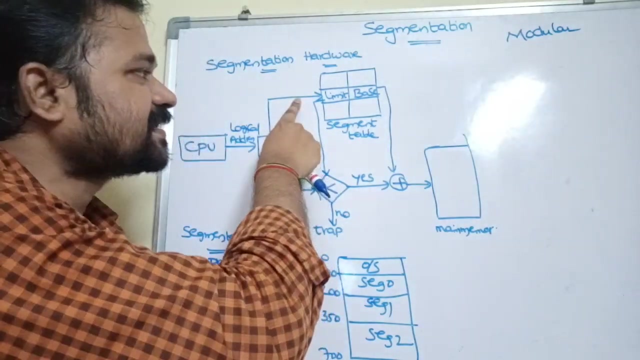 we can get the perfect area Segmentation. hardware CPU generates a logical address in order to execute an instruction, So the logical address is divided into two parts. The first part specifies segment number. The second part specifies offset. Offset means a location inside the, a location inside the segment. Here the segment number will be given as: 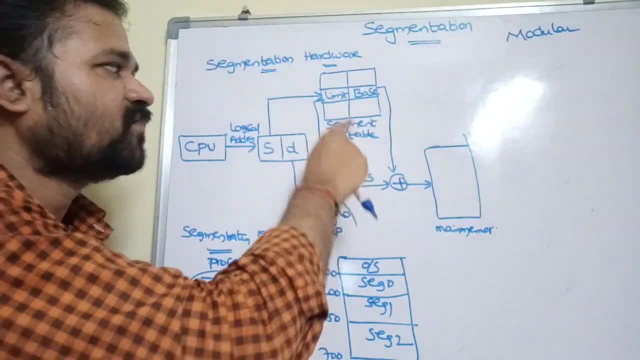 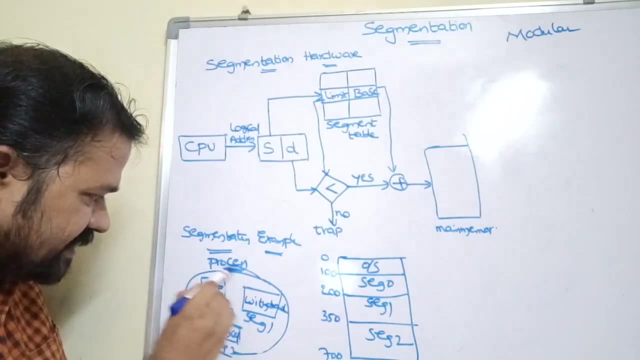 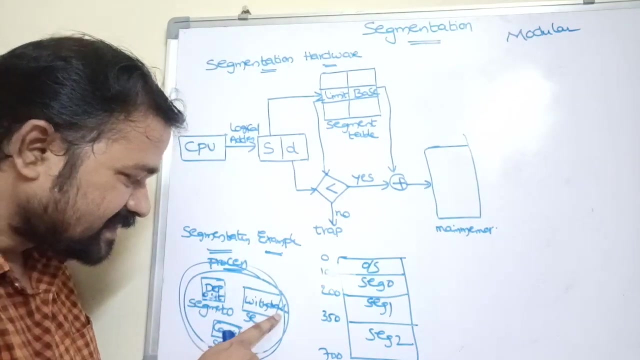 an index or input to the segment table. We know that every segment table contains base address and limit address. So let us see this example Here. this is our process. So our process totally contains three segments. The first segment is deposit. The second segment is withdrawal. 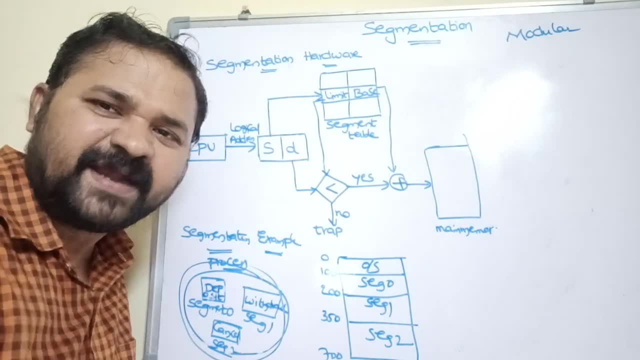 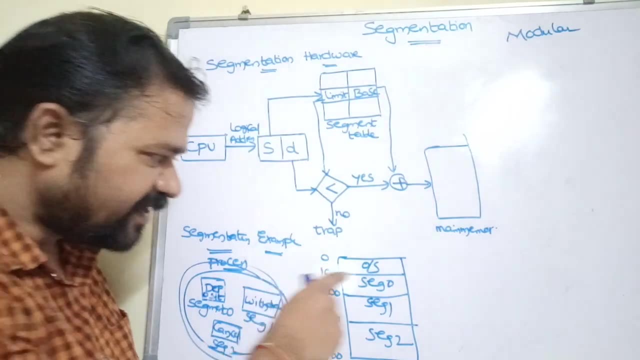 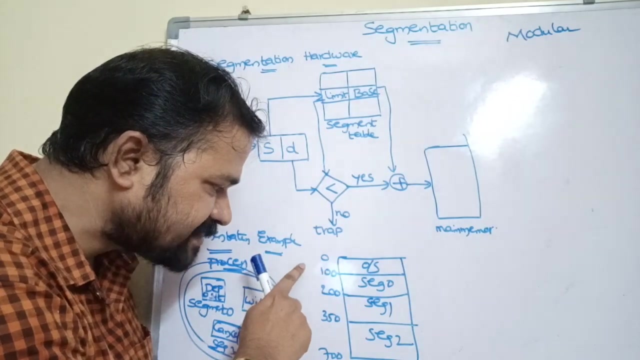 Third segment is some cancel account. Cancel Here, segment is nothing but a method only. So this is segment 0.. This is segment 1.. This is segment 2.. If you take the first part of the main memory is operating system. So this is segment 0.. For segment 0: what is the base address Base? 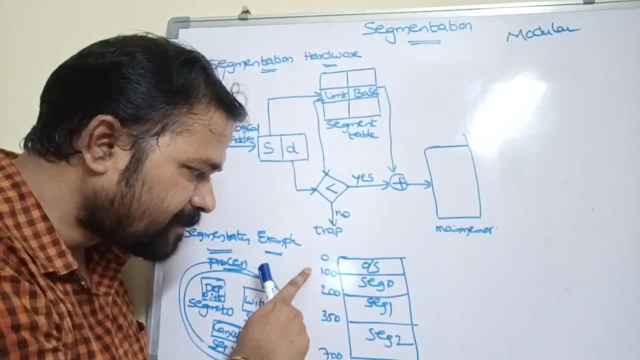 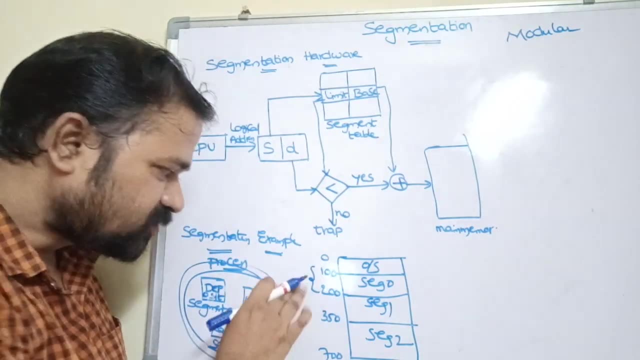 address means starting address of the segment. For segment 0 the base address is 100.. Where area, this limit specifies length of the segment. So what is the length of the segment? 100.. So let us assume that here CPU is accessing segment 1.. So what is the base address of? 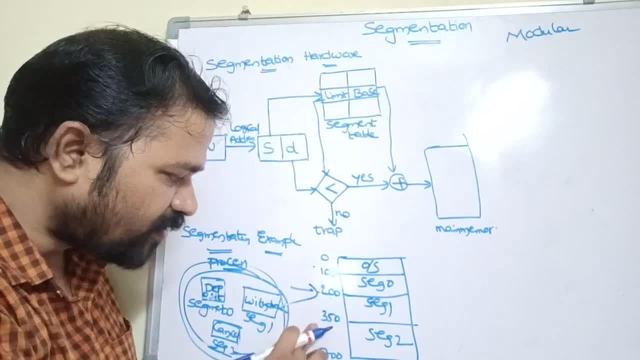 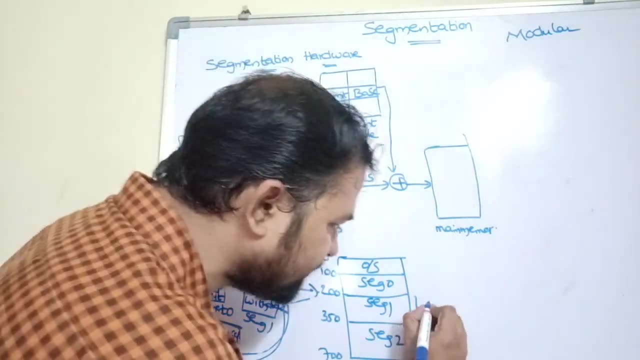 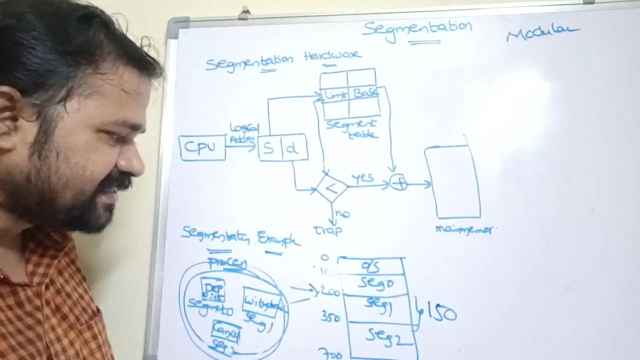 the segment. Here the base address is 200.. Whereas what is the limit of the segment? So 200, 350.. So limit means length of the segment. So 350 minus 200 means 150 is the limit here. So here, while accessing an instruction, CPU generates the logical address. 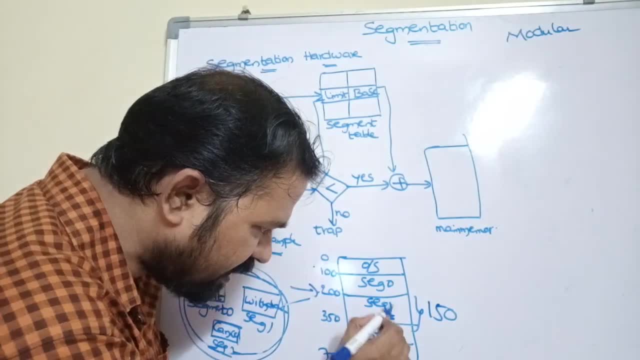 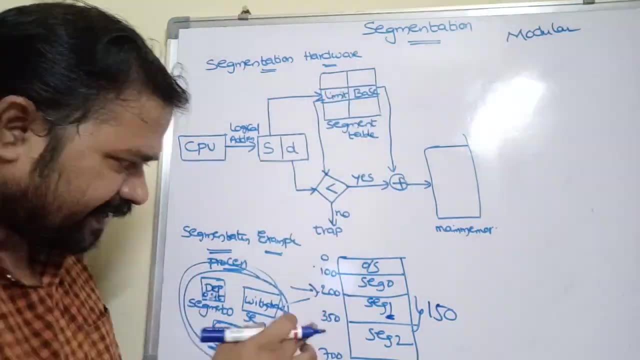 logical address contains segment number here. what is the segment number here? one. so this one will be passed over to the segment table so that we will get the base address and the limit address here. let us assume that the cpu is accessing segment 1. let here the offset is 50, what is? 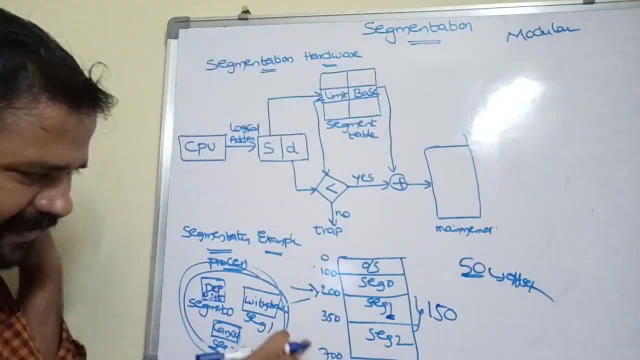 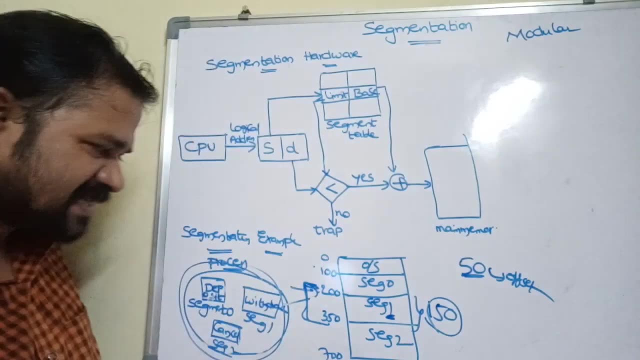 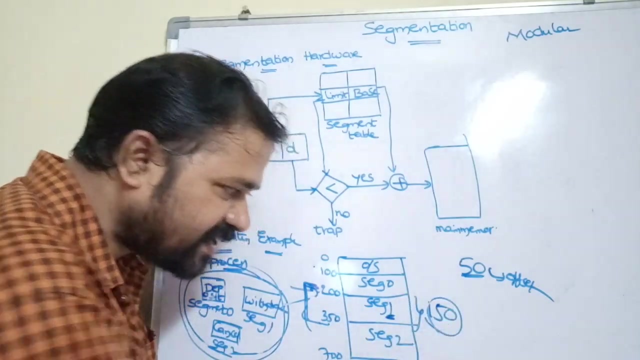 the offset here. 50 is the offset here. so here this 50 will be compared with length of the segment. offset means a particular location inside the segment. here how many locations this segment contains. this is the segment totally contains 150 instructions. so out of 150 instruction, which? 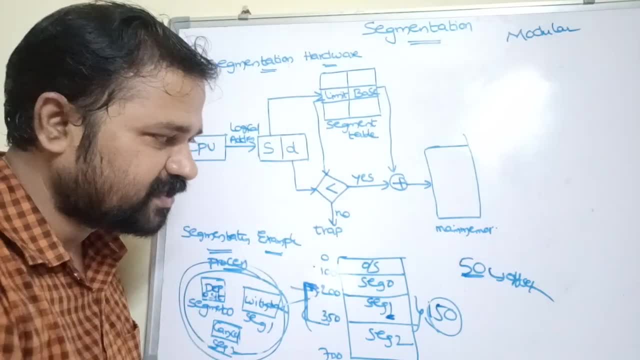 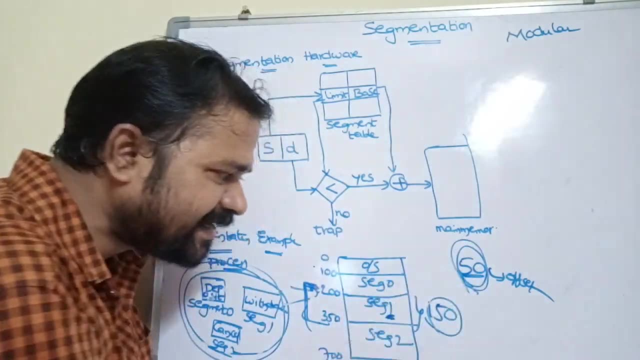 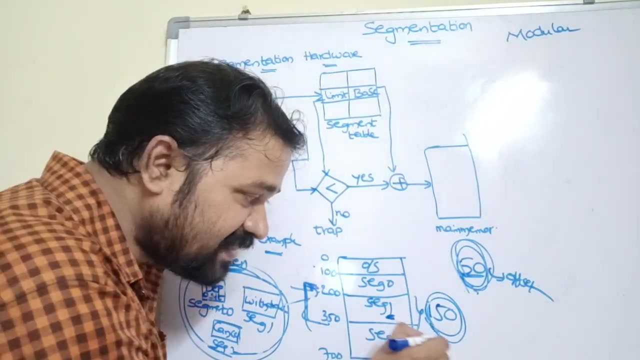 instruction we are executing that is nothing but offset, so that we are executing 50th instruction, so the offset is 50.. so we have to compare whether this offset is less than the limit or not. if this offset is less than the limit, less than the limit of the segment, so then only the segment is accessing the valid instruction. 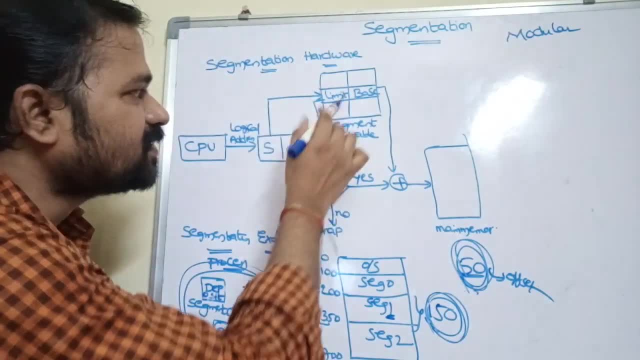 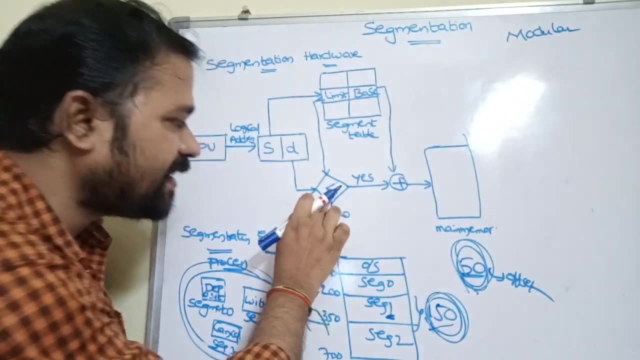 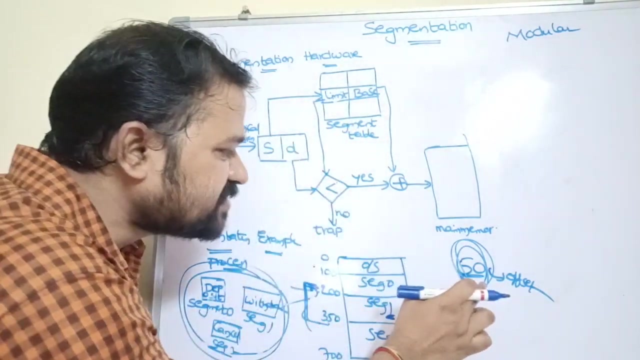 so here. so this is nothing but limit. so what is the limit of the segment 150? and what we are doing here? we are using a comparative less than comparator. so here we are checking whether this offset is less than the limit or not. here, what is the offset? here, 50 is the offset. what is the limit? 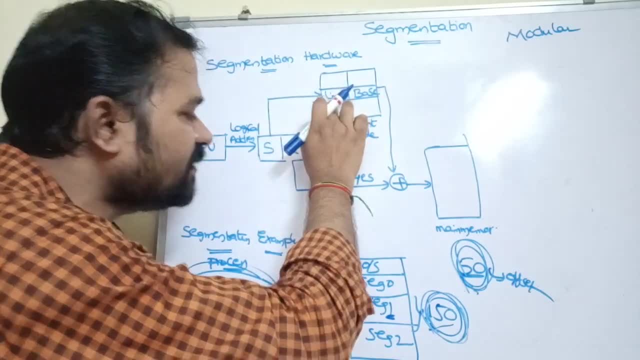 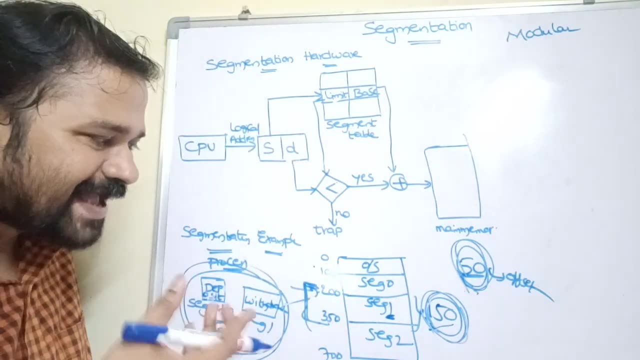 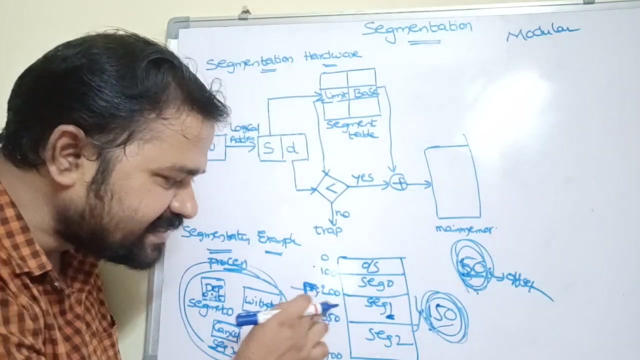 here 50 is less than 150, d is less than limit, so condition is true. so we have to execute the exact instruction in this segment. so how to get exact instruction here? we are executing 50th offset here, 50th instruction here. so that is nothing but 250. 50th instruction is nothing but here, the base. 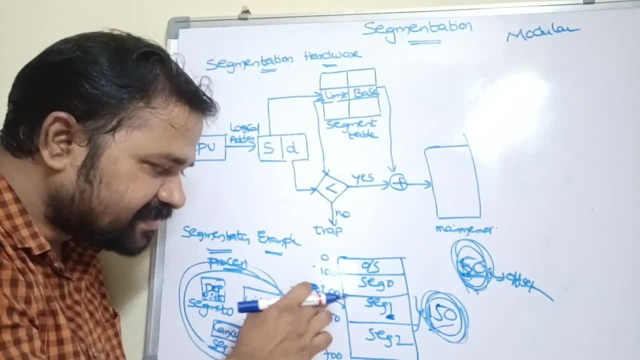 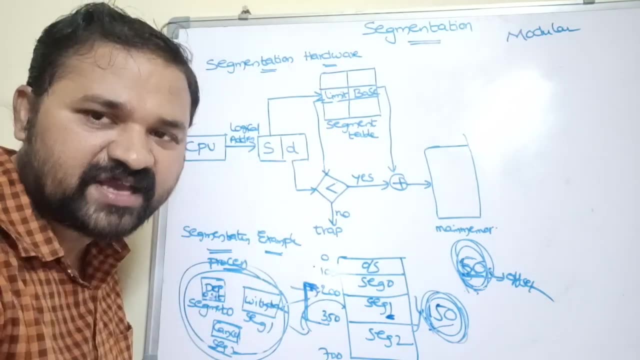 address is 200, so 250th instruction. so how to get 250 here? the base address is 200 where? So if we add 200 with 50, then it will give the exact location in the physical memory, main memory. So this is nothing but base address. 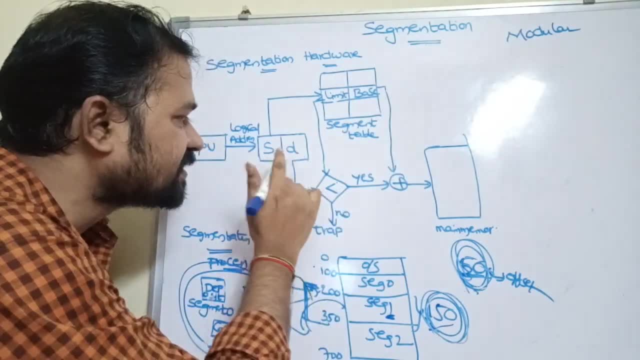 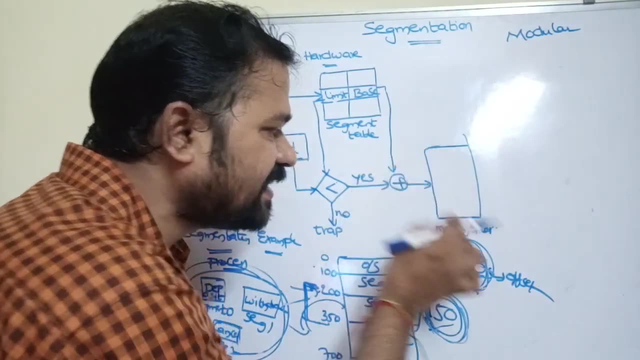 So with the help of adder we are adding the base address with the segment, So this D value and this base value are added together, So it will give the exact physical address in the main memory. So let us assume that here offset is some 200.. 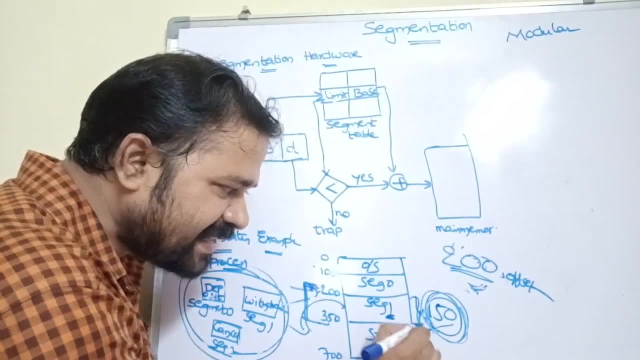 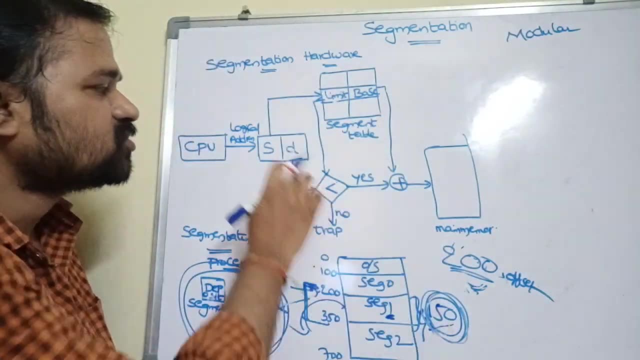 Let us assume that here offset is 200.. What is the length of the segment? 150.. So these two are compared here. So what is D value 200.. What is limit value 150.. So 200 is less than 150.. 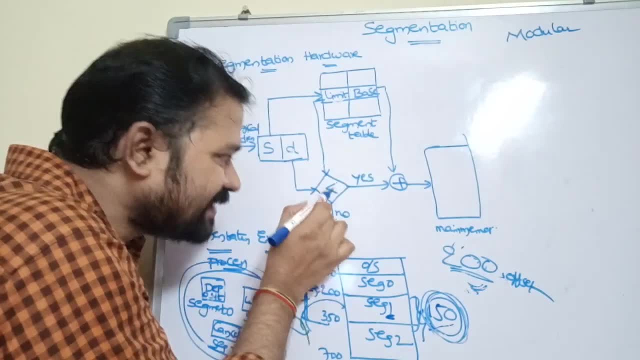 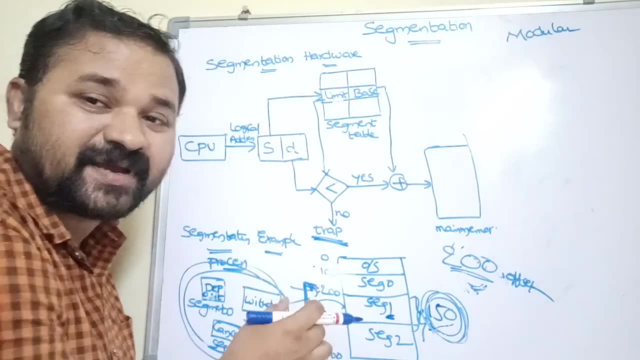 So condition is false. So what will happen? It will generate: whenever the condition is false, then this node will be executed. So operating system will generate a trap- Trap means interrupt- So that segment execution will be terminated. 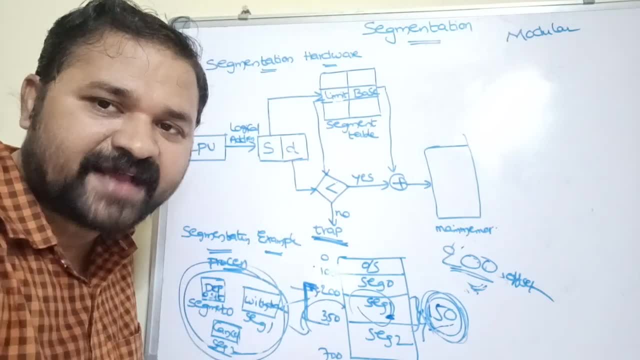 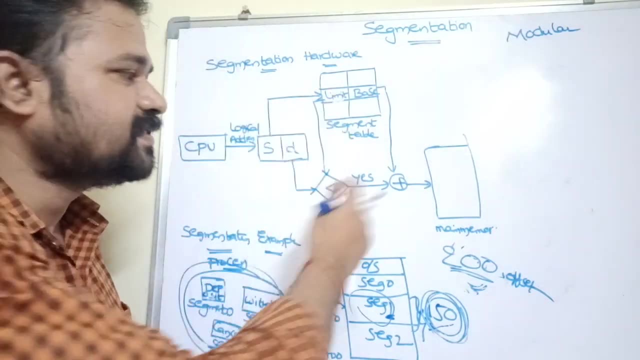 That means this segment 1 is trying to access other segments, So operating system generates the trap So that that process will be terminated. So this diagram is very, very simple. Let us see one more time. So CPU generates a logical address. 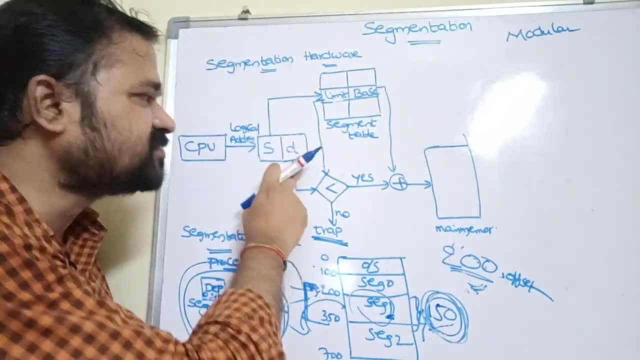 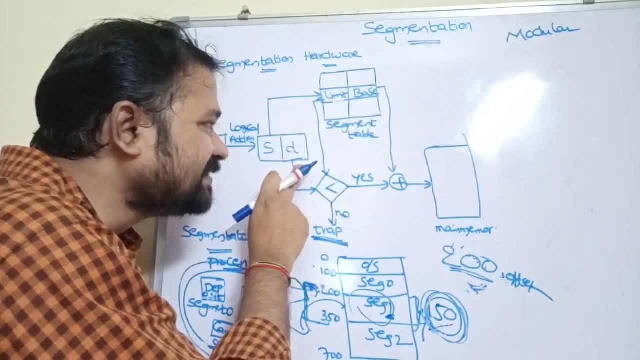 That logical address is divided into two parts: Segment number and offset. Segment number will be given as the input to the segment table. Next, with the help of the comparator, we have to check whether this offset is less than the limit of the segment or not. 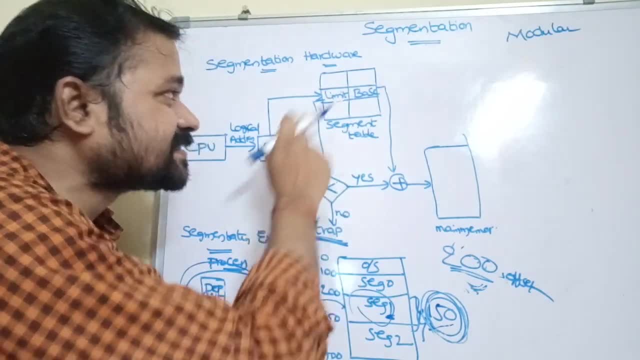 If this offset is less than the limit of the, if this offset is less than the length of the segment, If this offset is less than the limit of the, if this offset is less than the length of the segment, of the segment, then we can say that it is a valid instruction. So, in order to get the